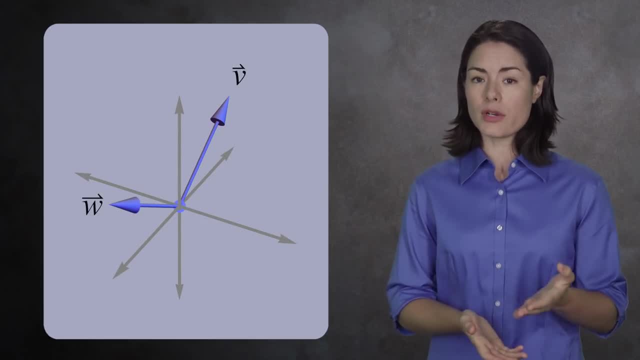 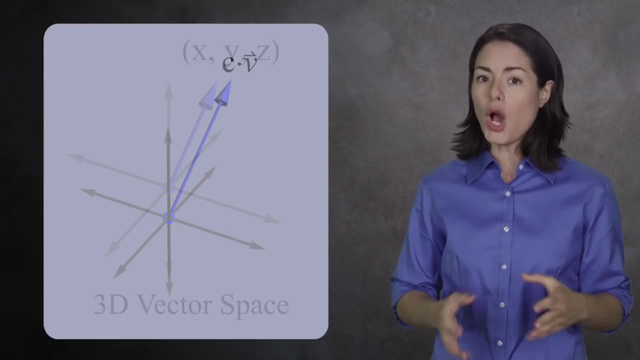 by the three coordinates. Like before, if you add two vectors in three-dimensional space, you'll get a third vector. And again, you can scale vectors by multiplying the coordinates by any real number. All of these vectors form a three-dimensional vector space, because 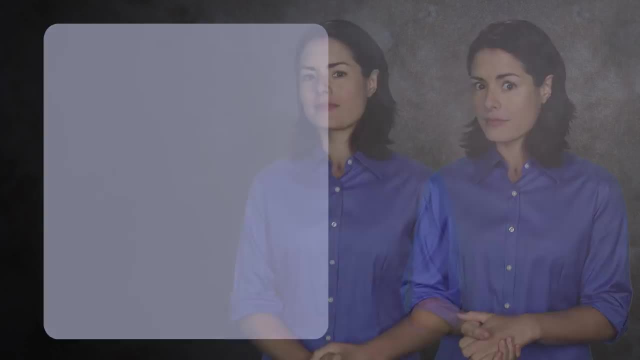 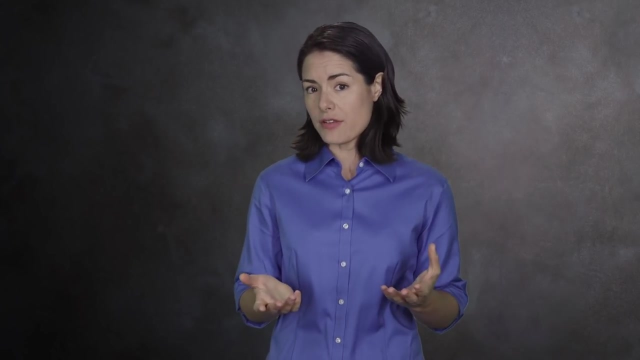 it takes three numbers to describe each vector. It's tempting to think that two- and three-dimensional vector spaces are all that we really need. Perhaps a fourth dimension is more important than a three-dimensional vector space. But, this is abstract algebra, and our goal is to generalize things as much as possible without sacrificing usefulness. 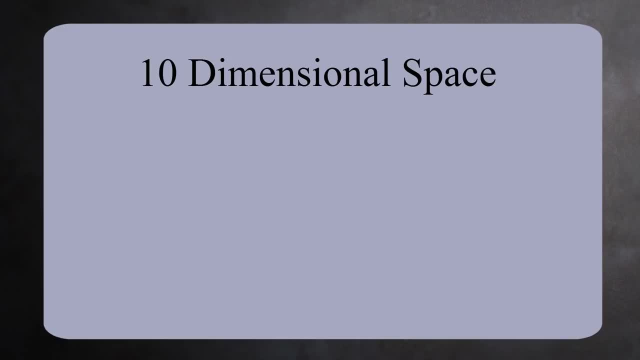 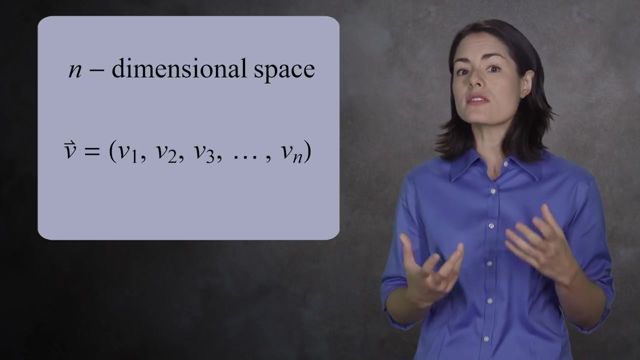 For example, imagine an alternate universe with ten dimensions. Taking inspiration from two- and three-dimensional vector spaces, we could suggest that in this universe, forces could be described by a list of ten numbers. And like before, you can add and scale vectors. We would call this ten-dimensional space. If you were to generalize this further, you could say n-dimensional space is a place where forces are described by vectors with n coordinates. We call this n-space. 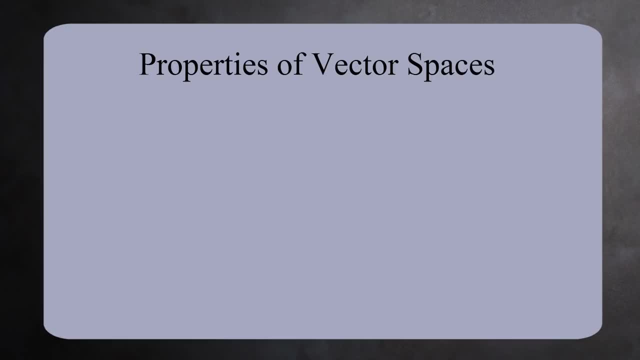 Let's stop for a moment and look at what properties all of these vector spaces have in common. For starters, you can add any two vectors, so there's an operation, addition. Better still, the order in which you add vectors does not matter. Vector addition is commutative. 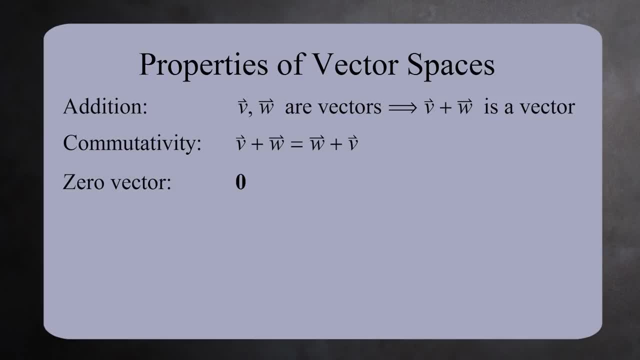 There is a zero vector, which doesn't point anywhere. So there's no point in adding any direction. Adding the zero vector to any vector leaves it unchanged. So the zero vector 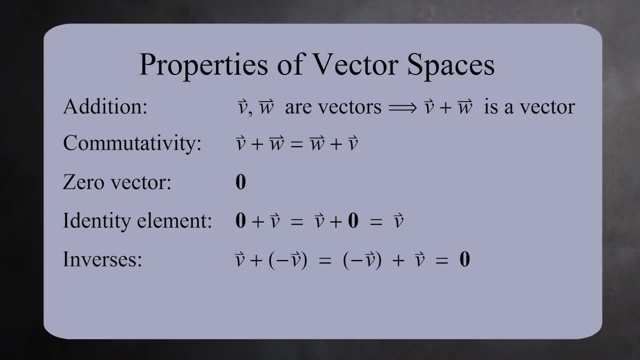 is an identity element. Also, for each vector, there is another vector which points in the opposite direction. When you add these two together, you get the zero vector. 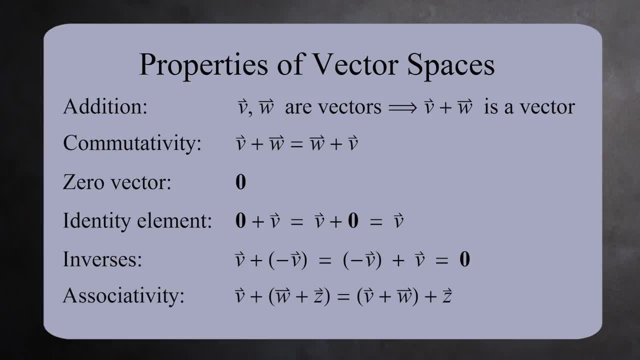 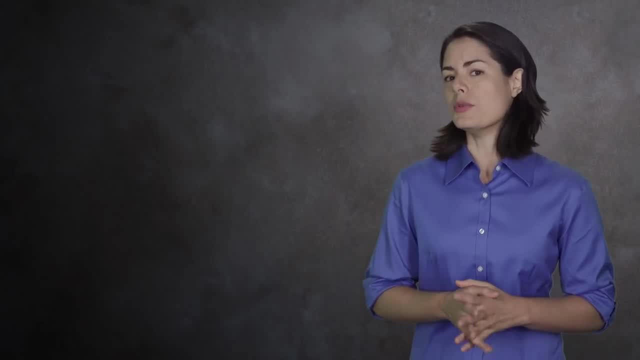 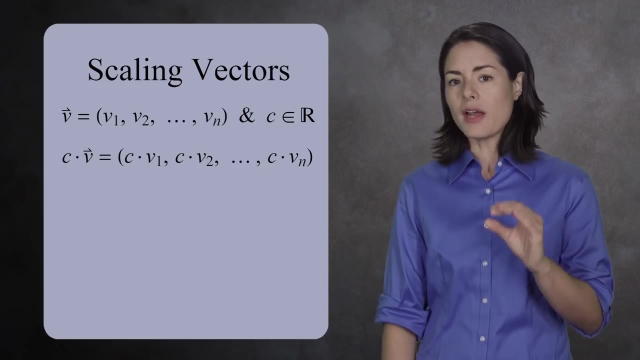 Vector addition is also associative. Taken together, we see that vectors form a commutative group under addition. But vector spaces are more than commutative groups. You can scale vectors by multiplying each coordinate by a real number. When you do this, the number 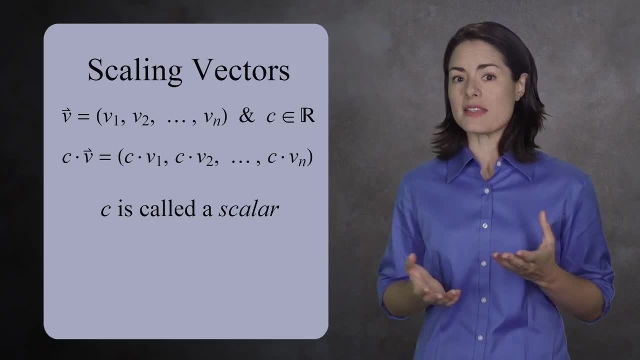 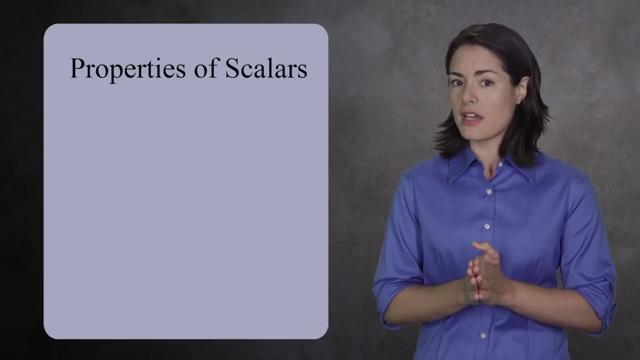 is called a scalar. These scalars give vector spaces additional structure and features beyond ordinary groups. And for the record, there are a few properties of scalars which will probably not surprise you, but they need to be said. Multiplying by scalars follows the 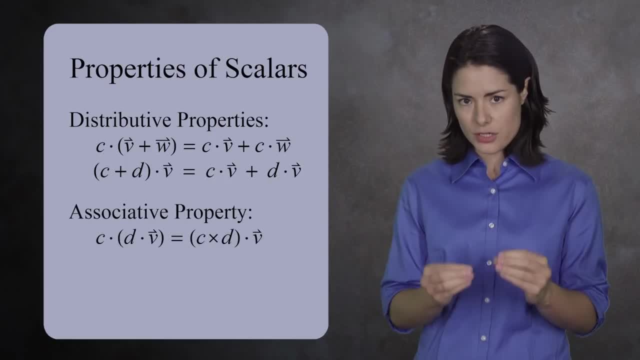 distributive properties. Scalar multiplication is associative, and multiplying a vector by one leaves it unchanged. 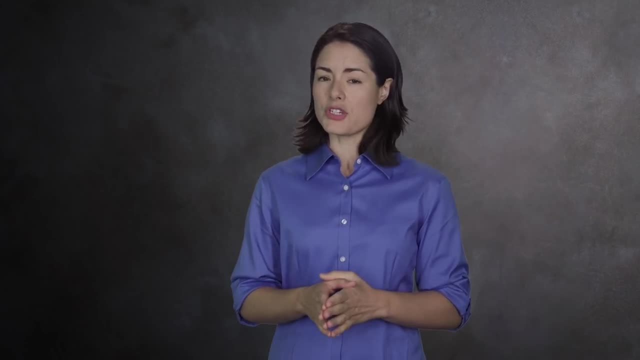 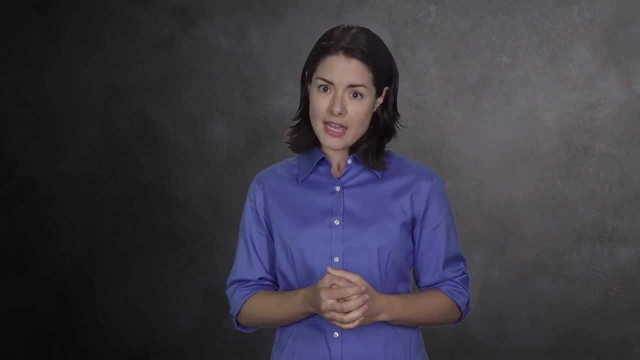 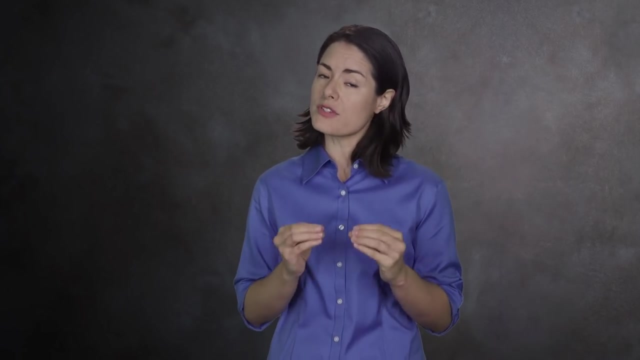 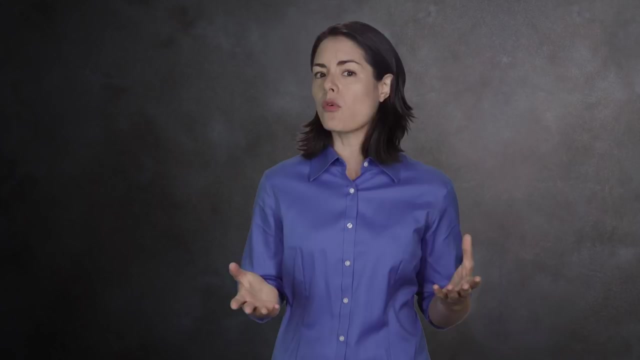 We're almost ready to give the textbook definition of a vector space. Up until now, we've thought of vectors as arrows in space. First, in two and three dimensions. Then, in any number of dimensions. We saw that in all of these cases, vectors were a commutative group with real number scalars. What if we took this as our definition of a vector space? Would it cover more ground than just describing forces in space? The answer is a resounding yes. 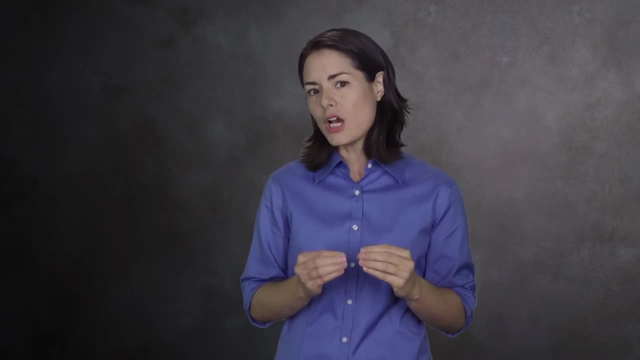 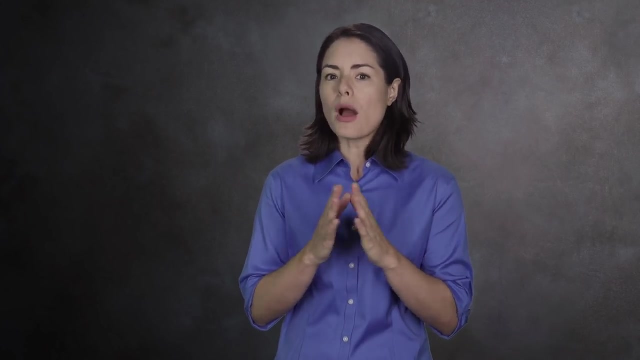 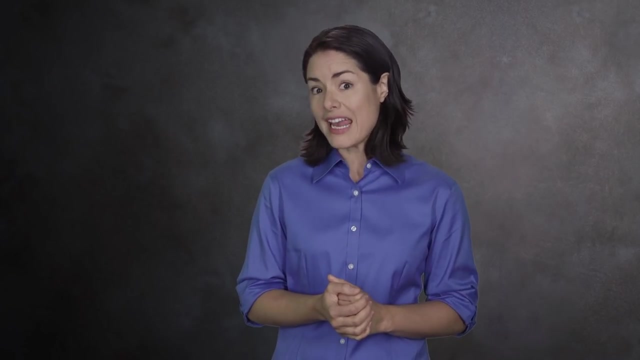 To get back from this idea that vectors have to have a physical meaning, we get something much more abstract, and much more powerful. And to take things even further, what if we threw out the idea that scalars have to be real numbers, and instead said they could come from any field, like the complex numbers? Now, we have a vector space. 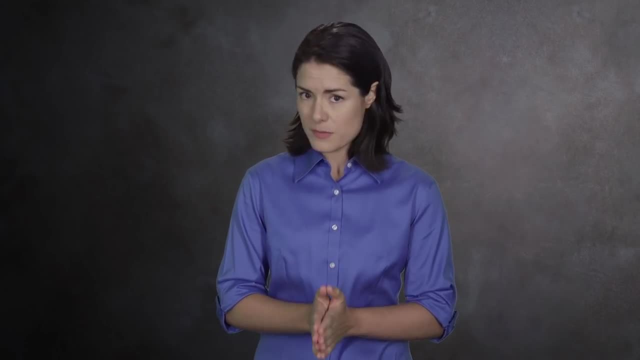 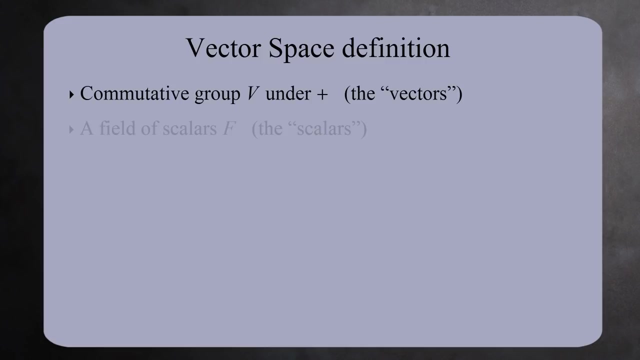 Let's take a breath and go over the abstract algebra definition of a vector space. First, you have a commutative group, and the elements in this group are called vectors. So, let's take a breath and go over the abstract algebra definition of a vector space. First, you have a commutative group, and the elements in this group are called vectors. So, let's start with a commutative group. Next, there's a field of scalars. You can multiply any vector in the group, by any scalar in the field, and you'll get a new vector. The operation between scalars and vectors obeys the distributive and associative properties. And lastly, vectors are unchanged when multiplied by one. Here, we have the full definition of a vector space. 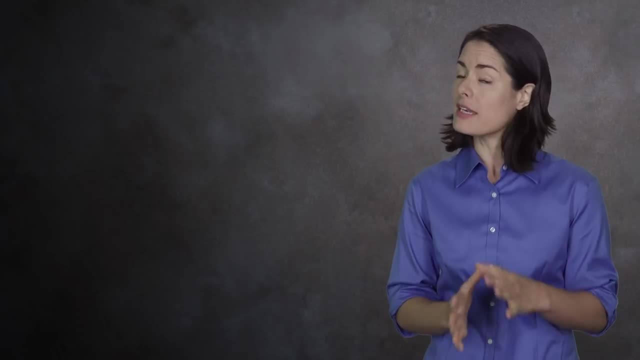 As mentioned earlier, this more general definition encompasses many more situations. Let's see 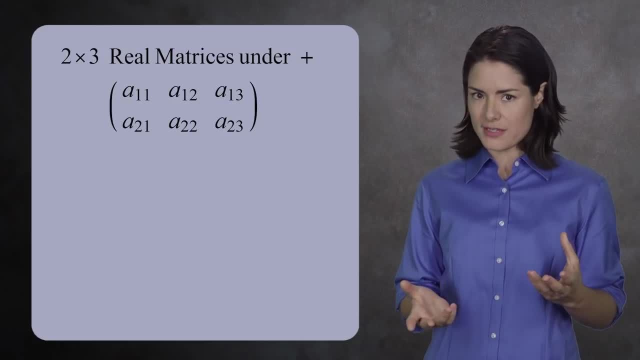 For example, consider all 2x3 real matrices. These matrices form a commutative group. 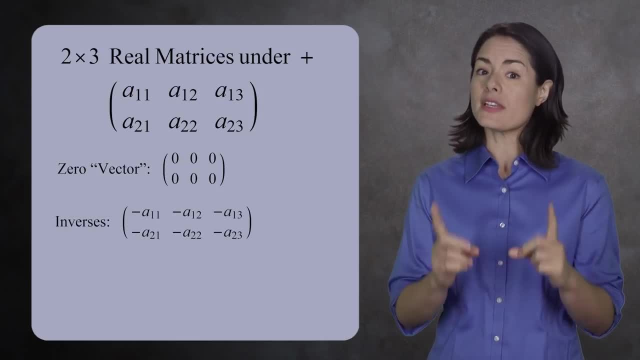 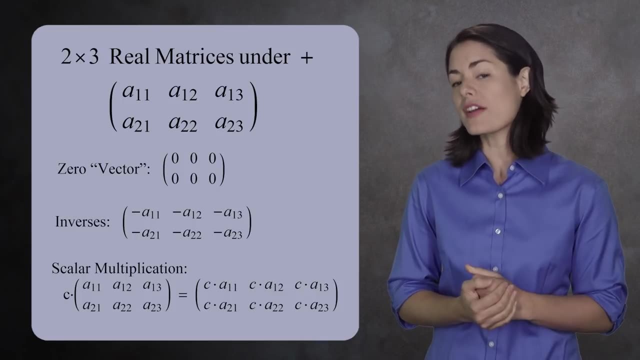 You have a zero matrix, inverses, and you can even multiply any matrix by a real number to get a scaled matrix. The 2x3 real matrices form a vector space, and it's a good exercise to check the remaining properties. 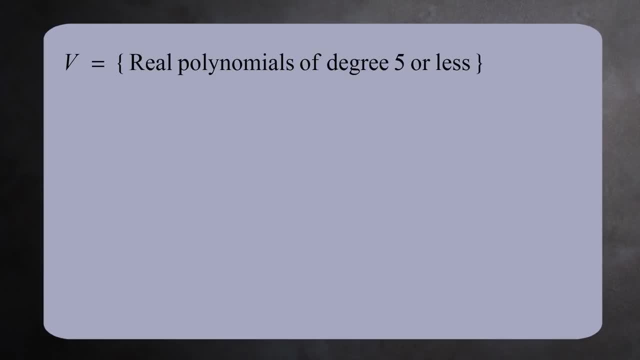 For another example, consider all polynomials with real coefficients of degree 5 or less. This set also forms a vector space. If you add two polynomials of degree 5 or less, you'll get another polynomial of degree 5 or less. 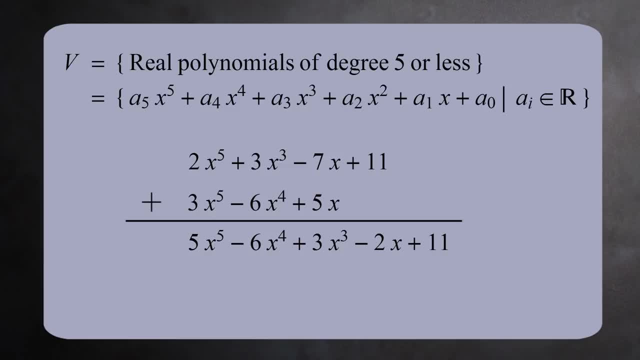 And notice how I keep saying, or less? This is key. 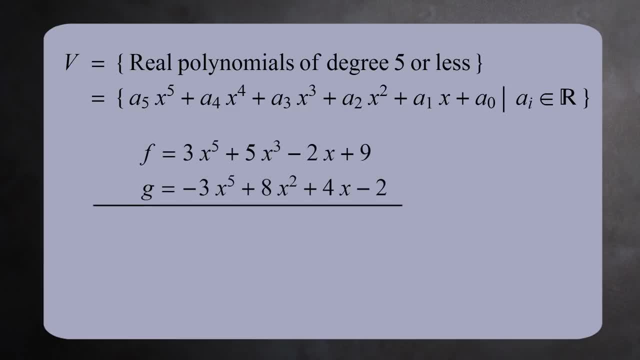 Look what happens if you add these two polynomials of degree 5. You get a polynomial of degree 3. So when you add two polynomials in this group, the degree may go down, but it will never go up. 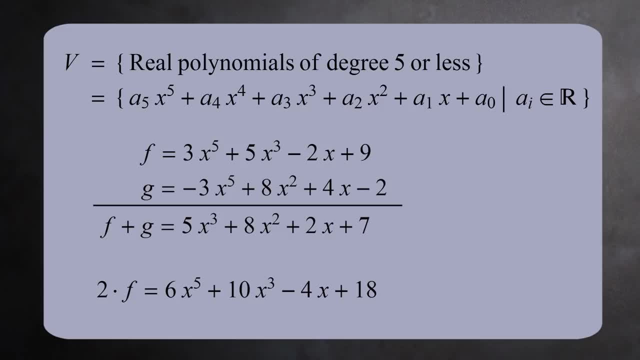 And once again, you can multiply any polynomial by a real number. And get another polynomial of the same degree, unless you multiply by zero. Let's see one more example. 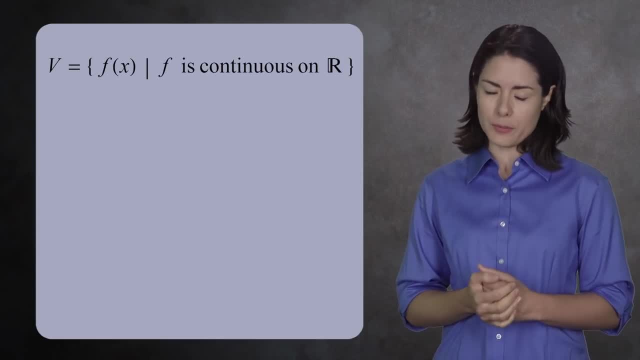 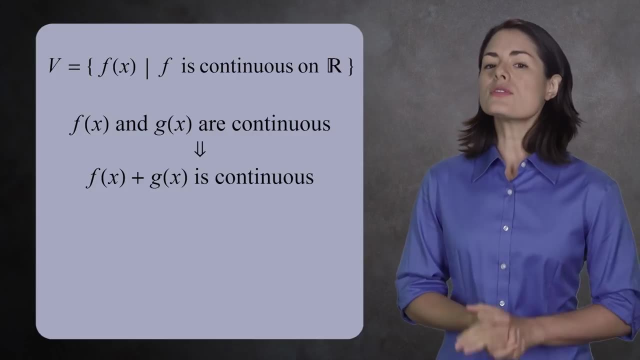 Consider the set of functions which are continuous over all real numbers. In calculus, you learn that if you add two continuous functions, you get another continuous function. It's also good practice to check that multiplying a continuous function by a real number doesn't cause any problems. 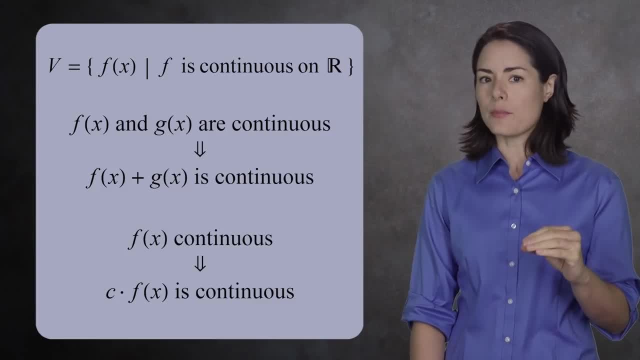 It's still a continuous function. This is a great example of a vector space. That really departs from the original idea of arrows in space. 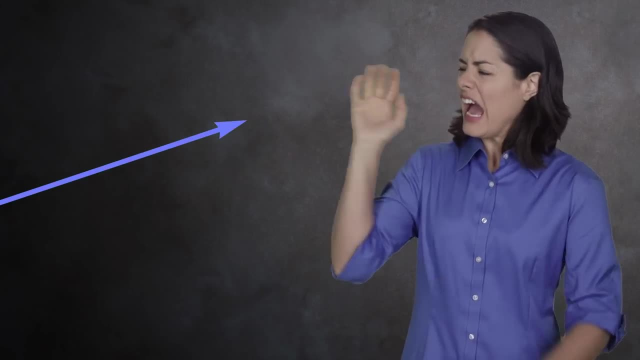 Vectors can be pointy things. Ow! 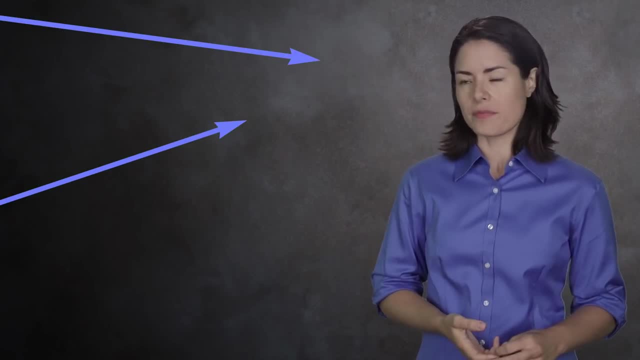 I'm not sure what these vectors are pointing at. Hog in計接下來. W-m-x-3 y-u-f-u-r-h-h y-ho-w y-p-anda w-m-a-n-t w-b-n-e-d i-o-a qy-a-c-i-a-n-a-n-o-0 w-i-n-2 y-a-t-v-a-v-er-v-a-t-h-i-a-s-t i-n-4 w-p-i-n-e-n-k-o-n-a-t-i-a-n-n-s-a-n-s, 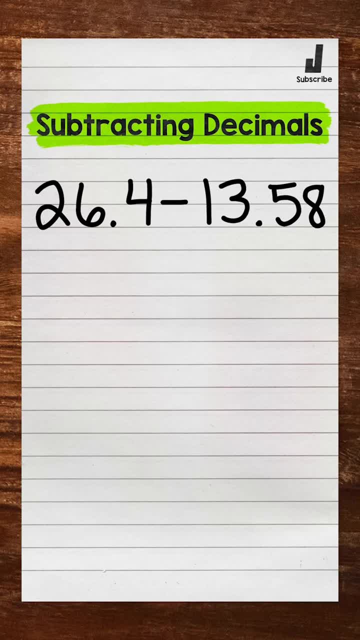 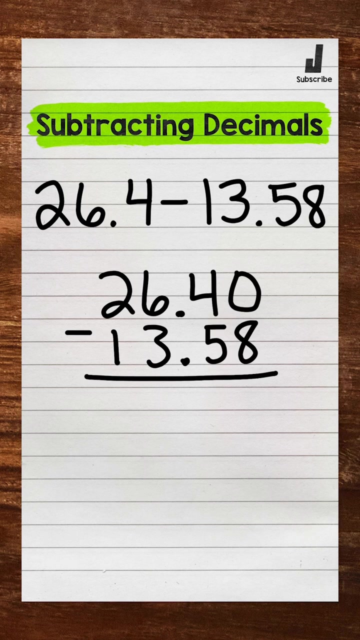 This is math with Mr. J. Let's subtract decimals. We have 26 and 4 tenths minus 13 and 58 hundredths. Let's set this problem up. We do that by lining up the decimals. Now the problem will look a little offset, but we can use a placeholder zero. That way both decimals go to the hundredths place. Now we subtract 0 minus 8. We need to borrow. So we have 10 minus 8, which is 2. Now we have 3 minus 5. We need to borrow again. So we have 13 minus 5, which is 8. Bring the decimal straight down. And now we have 5 minus 3, which is 2. And then 2 minus 1, which is 1. So we get 12 and 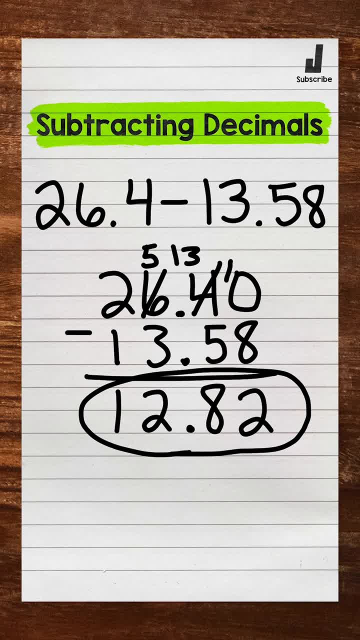 82 hundredths. So there's a very quick review. Check the description. 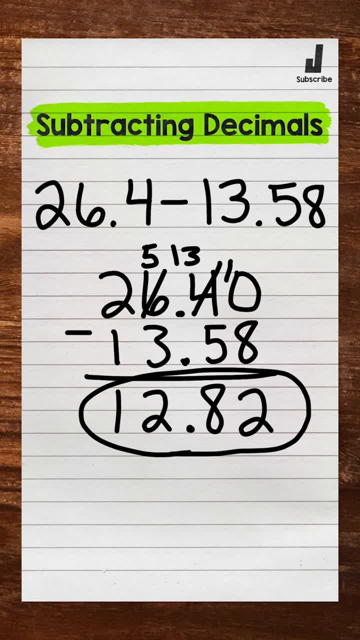 for a link to a more detailed explanation. Until next time, peace.